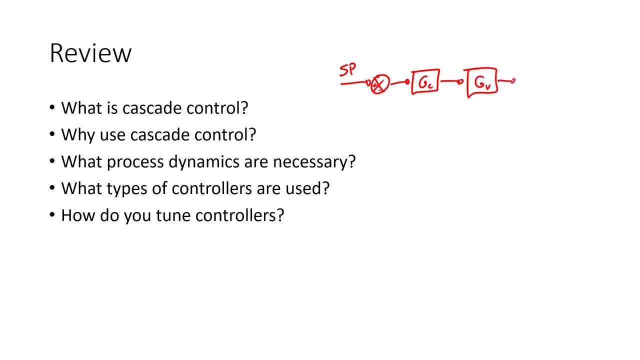 maybe a final control element like a valve, and then I have my process, And this is going to be my process variable, and I might have a measurement dynamics as well. So this is a standard feedback control loop. One of the things that we're going to be looking for are disturbances that are going 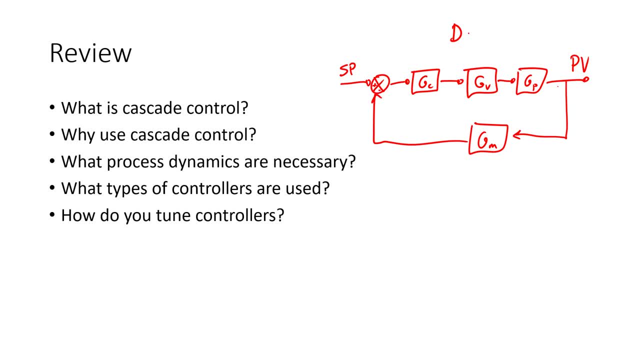 to affect our process. So I have a disturbance that you know I can either measure or not measure and that's going to affect my process. Okay, I'll just add that in Right there it drives me away from the set point and then I have an error between my process. 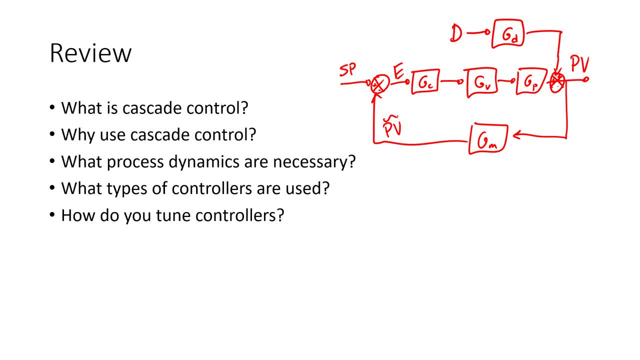 variable, my measured process variable and my set point, And then my feedback control loop is going to then take care of that error. But let's say we can measure the disturbance or measure the effect of the disturbance, and we want to reject it before it causes me to have an error in my system. 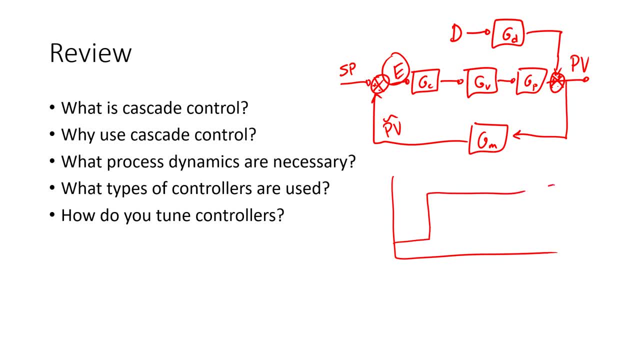 Just as a graph, I'm going to have a set point. Okay, and let's say there's my process variable and I have a disturbance that repeatedly brings me away from that set point. Then can I do something with my manipulated variable? Okay, here might be my manipulated 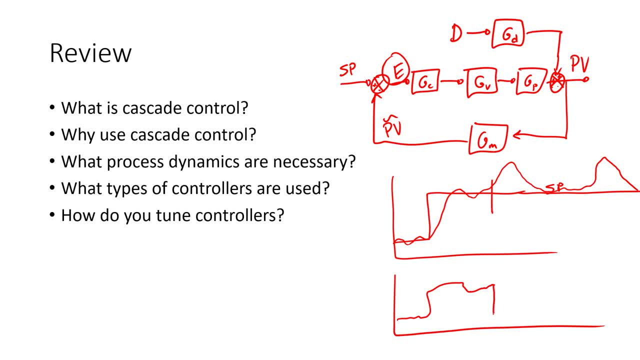 variable right at this point, when I measure that disturbance, to counteract it in some way, so that the disturbance is not going to cause me to have an error in my system. So I'm going to add that, Okay, and let me add an error into my system and add a sequence of errors again. 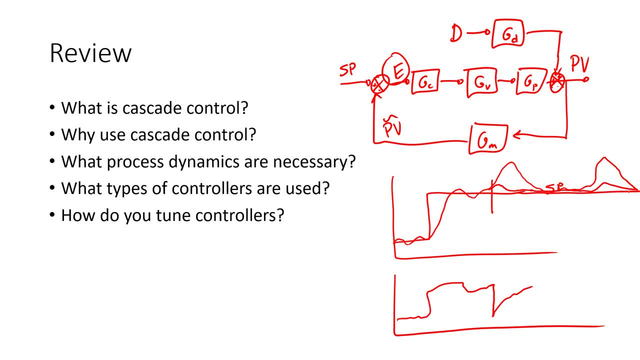 All right, all right, please. Okay, here you see that I've created what's called a surface, and I'm not assuming that pleasure. And then let's just leave it for the moment. Whoa, What did we call it again? Oh, what did we call that again? Oh, we did the same thing for. 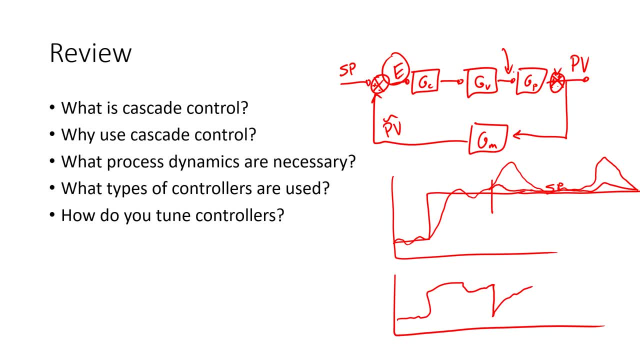 winter parentheses, and then plus minus, Oops. so one step. we're gonna finish that up units once the stage is completed, Okay, So we're gonna're trying to put this strings together and we're finally back to work. then you're able to achieve better control, okay. so what we're going to do is we're going to erase 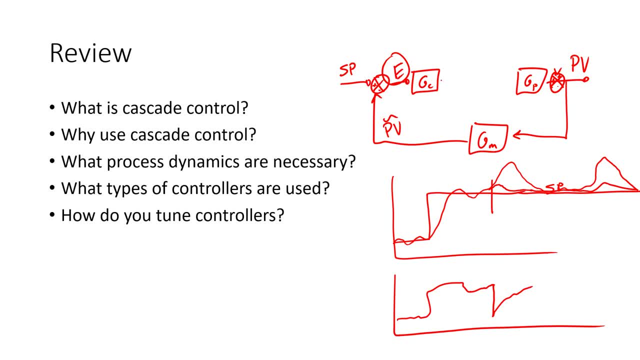 some of this and we have this controller. this is the- we'll call this the master or the outer loop controller. that's going to provide a, a set point. that's going to provide a set point to the inner loop. okay, and then i'm going to have another plus minus, and then i'm going to have a second. 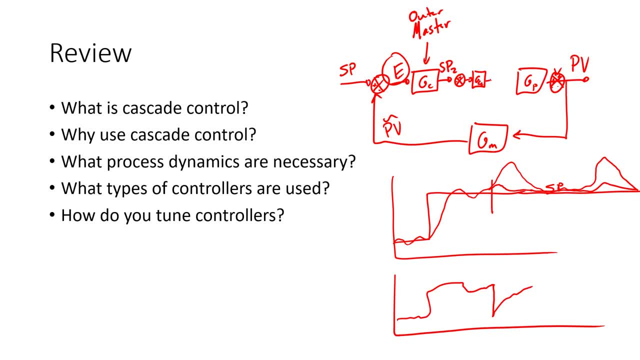 controller, okay, and then that is going to change the valve, and then i'm going to have something like a flow, but i'm going to have a feedback there. okay, there's my minus there and my plus, okay. so this is an inner loop right here and that's. 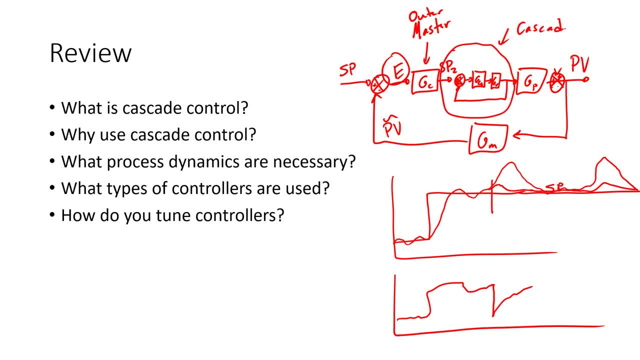 some of the inner loop that i've got here and that's the inner loop. so i'm going to. we have a cascade. We call it a cascade because the outer is giving a set point to the inner and we're cascading these set points down. Okay, so we're also going to talk about the 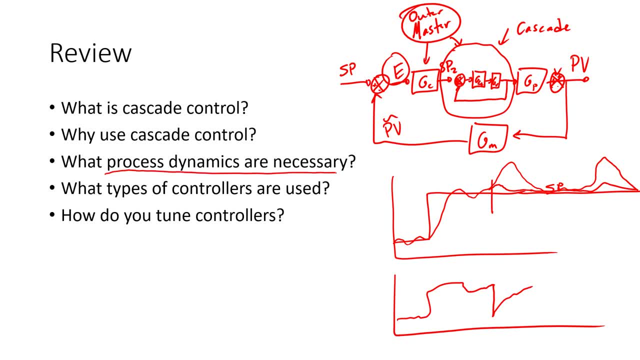 process dynamics that are necessary. You know, this inner loop, right here, has to be much faster than the outer loop. Okay, so we typically want it to be about three times faster than the outer loop in terms of following the set point, And we'll show you an example of 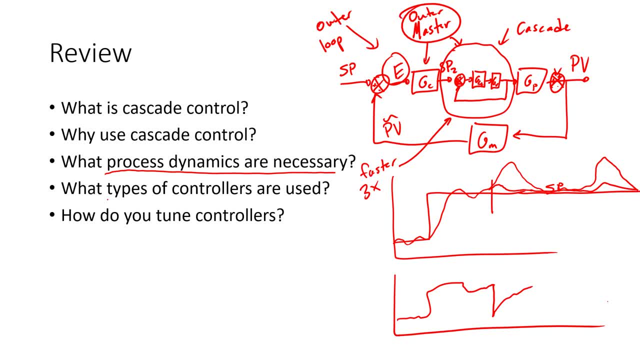 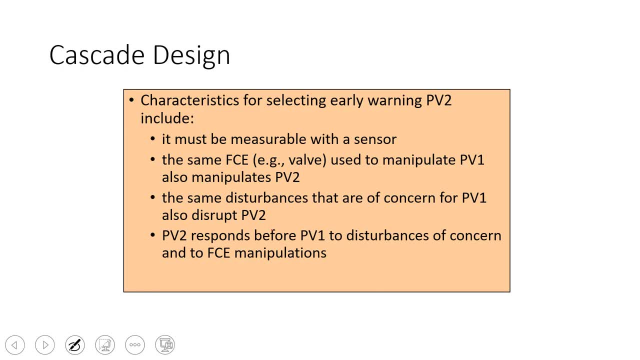 why that's the case. So what types of controllers are used? We'll talk about that. And then how do you tune these cascade controllers? So, first of all, cascade design: Characteristics for selecting this early warning. you know, in this case it might have been that. 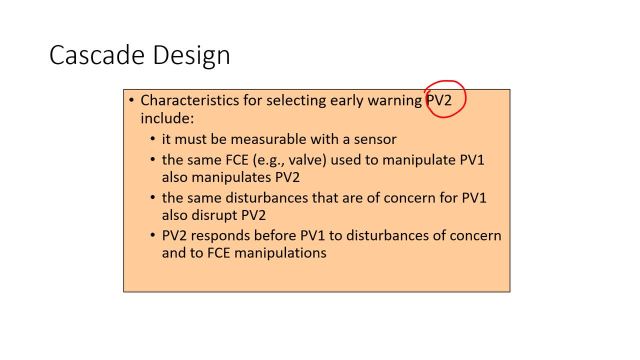 flow. It has to be measurable with a sensor. So we're adding an additional sensor to our feedback controller and we're setting up an inner feedback loop. We also have to use the same final control element, for example, in a valve that's used to manipulate this outer loop. 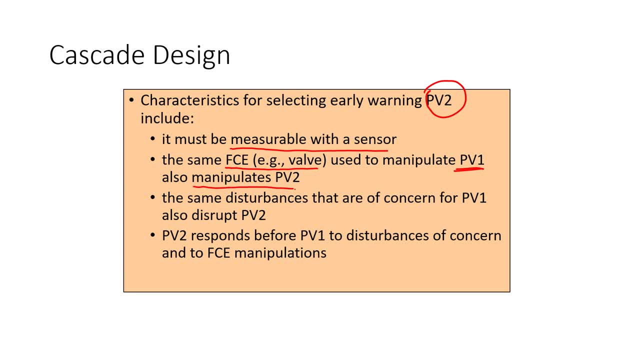 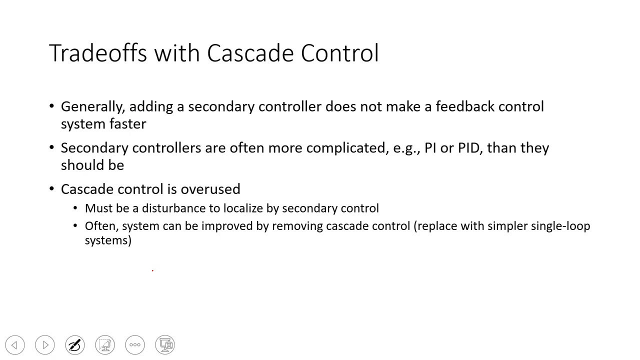 PV also manipulates the inner loop PV. Okay. so the same disturbances that are also of concern for PV1 also disrupt PV2.. And then we need PV2 to respond to the set point changes of the inner loop much faster than the outer loop. Okay, so here's some trade-offs or misconceptions problems with. 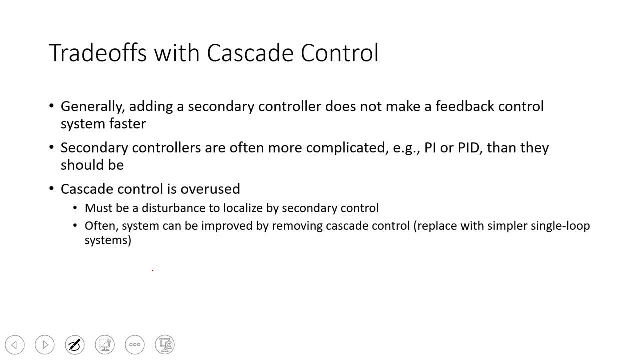 cascade controllers Generally. adding this secondary controller does not make the feedback control system faster. It's just going to reject frequent disturbances that might be affecting the process. Also, the secondary controllers are often more complicated Once you start adding cascade layers. this whole feedback 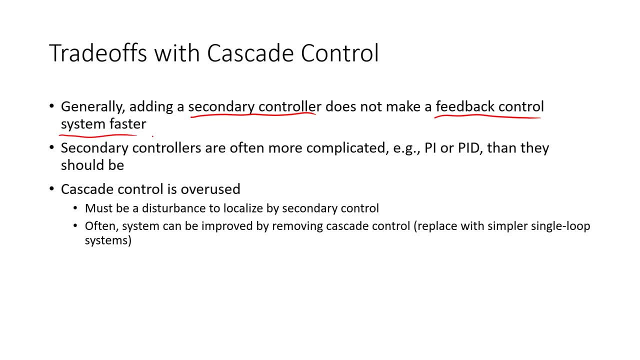 control often becomes much more difficult to maintain and tune, And that's just an added layer of complexity that you're adding to the system. Just an observation is that cascade control tends to be overused. Okay, we tend to build in complexity as different events 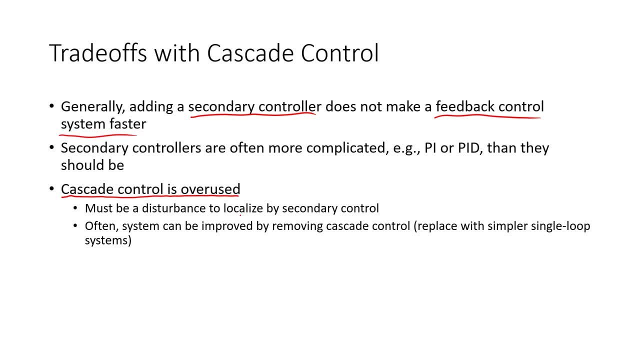 happen in control systems and it's easier to add things than to take them out. Okay, so sometimes a system can actually be improved by just removing these layers of cascade control with simpler single loop systems. So just some things to watch out for out for. on cascade control also, you know common cascade controller that you see. 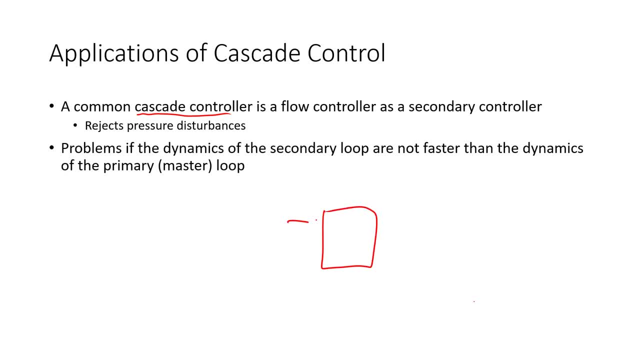 very frequently. let's say you have a tank reactor, for example, and you might be trying to maintain a temperature in that reactor. okay, and I'll put a temperature controller, and you know. let's say we want to adjust, you know, the flow coming into the reactor- let's say reactant or something like that. you know. 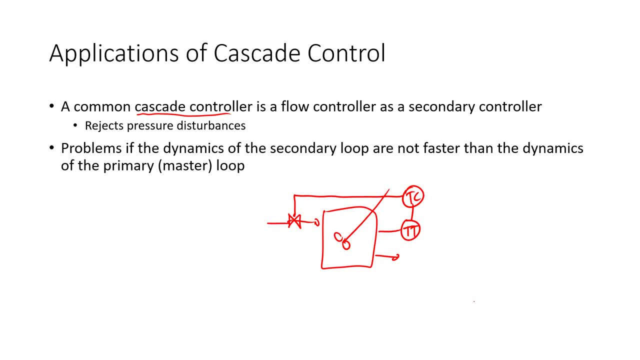 this is. this would be a common feedback control system, and what we're going to do here is, if we have, for example, a Delta P, you know pressure change from the inlet side, you know, maybe that fluctuates with time. that's a disturbance. so the same valve position gives me different flow rates. I can add a flow transmitter and 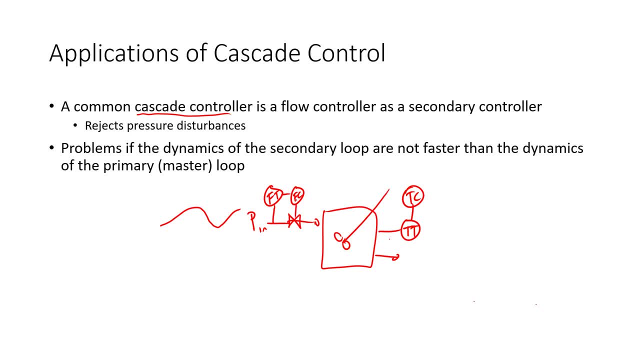 then set up a flow controller that's going to maintain that flow that we requested. and now the temperature controller: instead of writing directly to the valve, it writes a set point to the flow controller. so this is a cascade controller. so let's go back and look at the control structure. this is the master. 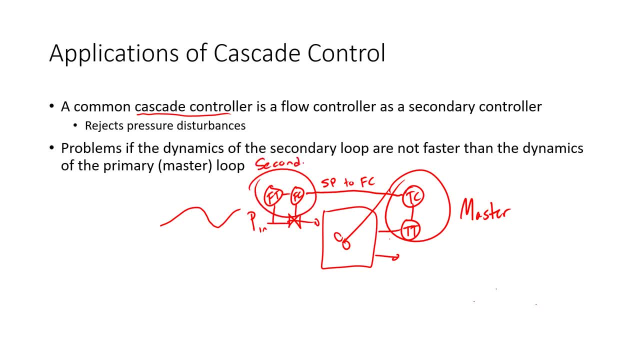 right here, and then this is the secondary control loop and then we'd also call this the primary. okay, so the really important thing here is that you can have a lot of problems if the dynamics of this secondary loop are not faster than the dynamics of the primary master loop. 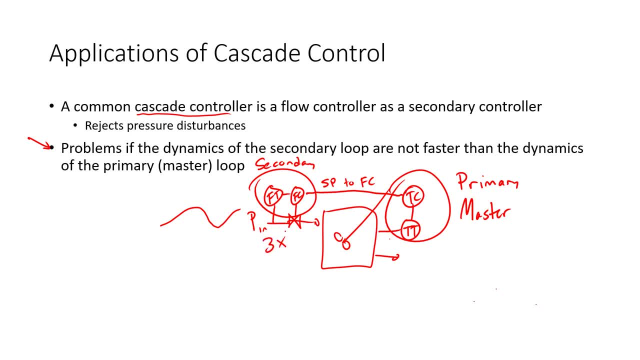 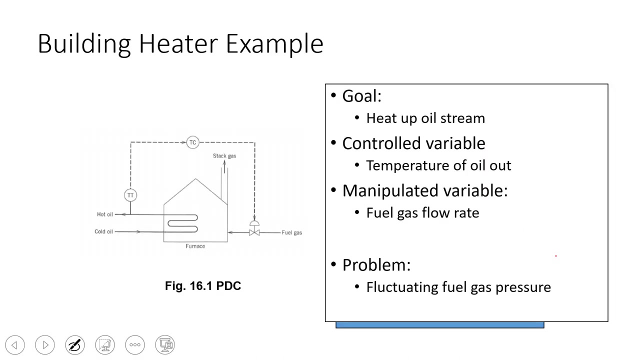 this takes. you know that we need this to be about three times faster to reach the set point than the master is requesting. so sometimes we even have to detune or slow down the the master controller so that we don't keep changing the set point on the secondary before it can respond okay. so here's a. 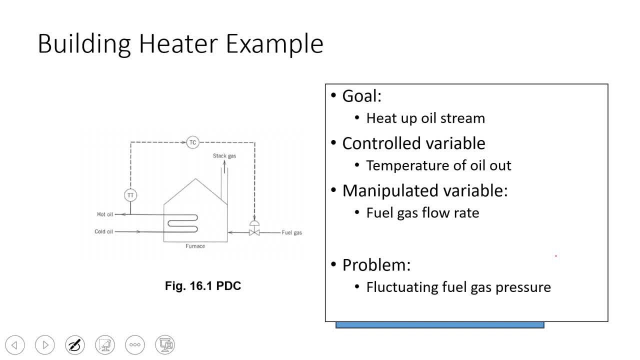 building heater, example, and the goal is to heat up an oil stream. okay, this, right here we're trying to maintain a temperature coming out of this furnace. so you know we have a flame here. and then stat gas. okay, we have, you know, this fuel gas coming in right here. that's providing. 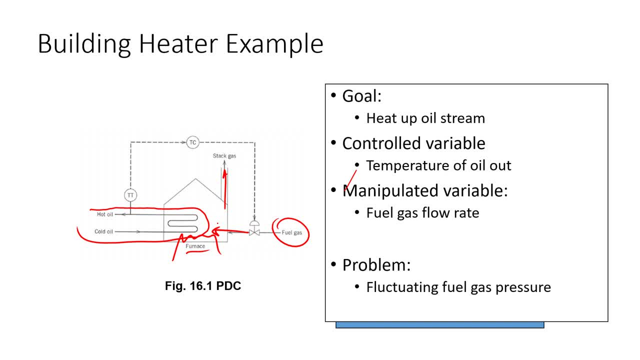 the ignition, or, sorry, the fuel for the, the flame, and we have a little bit more coal up and we have this來了 a temperature. we want to maintain this at a certain temperature. we might have a set point, you know temperature set point, maybe that's, you know, a thousand degrees. 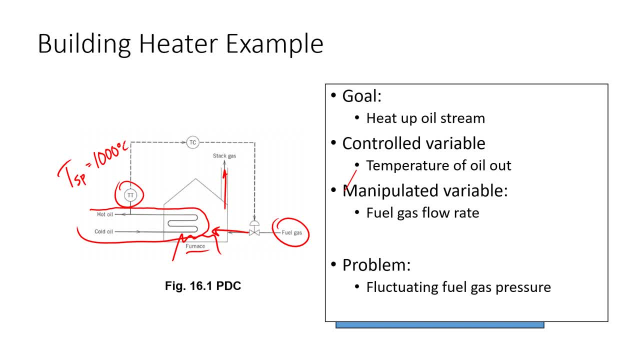 Celsius, for example. you know, whatever that might be okay. so if it's too low, it's gonna open up this valve a little bit more, so that might be the valve position versus time in order to maintain a temperature set point. okay, so if I'm too low and opening up that valve is going to increase my 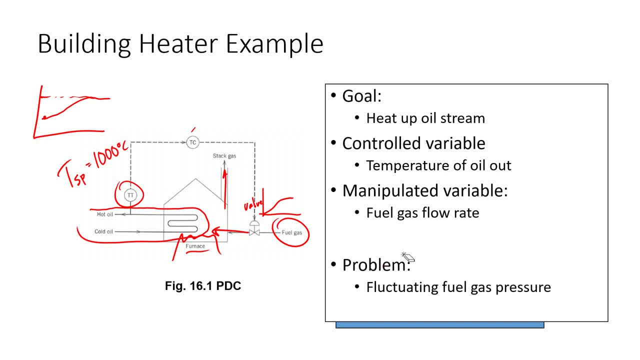 temperature. okay, so we have a couple things here. we have the controlled variable is my temperature of oil out. my manipulated variable is my flu fuel gas flow rate and I'm have a problem here, a fluctuating fuel gas pressure. so this is my pressure of my fuel gas supply and that is. 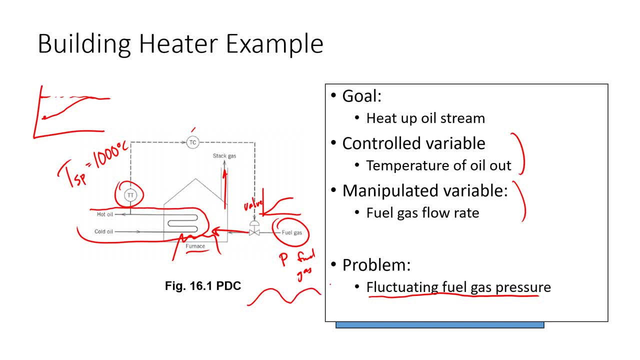 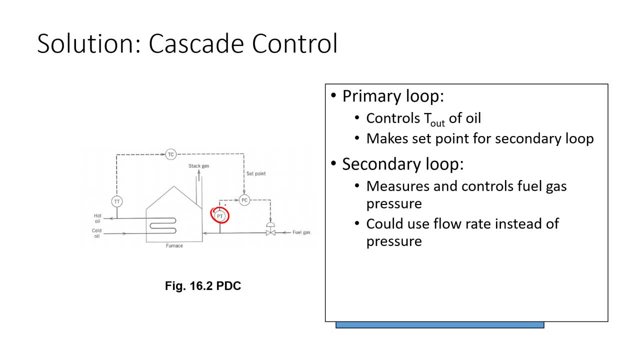 fluctuating, so one solution is cascade control for this. so if we want to measure pressure right here now, this could also be a flow controller. so, for example, if I just change this to an FT and an FC, install a flow transmitter, flow meter there and then have a flow controller that might be more common than a pressure one. okay, 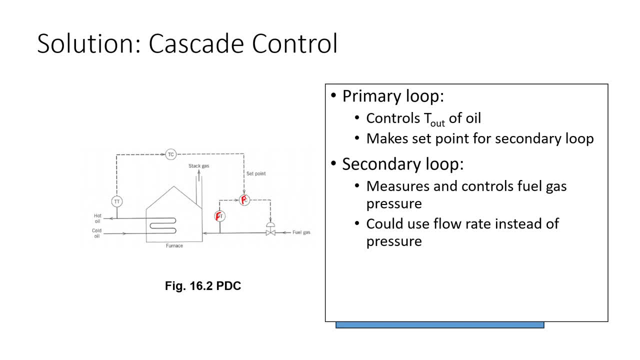 so primary loop consists of the temperature out of the air and the oil, and this makes a set point for the secondary loop. and then the secondary loop measures and controls the fuel gas pressure, and this is a set point. okay, this is going to be a set point to the secondary, okay, so let's take a look at. 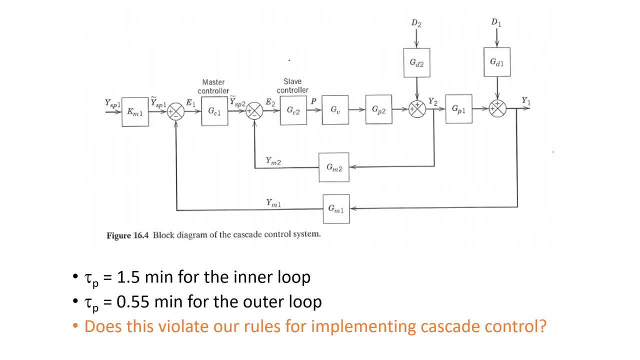 an example here: we have this secondary controller right here and the primary right here. this might be our flow controller, for example, and this might be our temperature. okay, so let's say we characterize the inner loop and we have a set point change on the this inner loop, this would be a flow and this would be my set point. and then 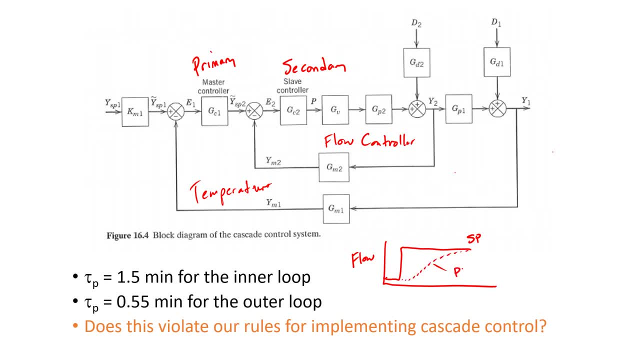 my PV value, my process variable value, and let's say this takes for about 63% of the way to get to the new set point. it takes about 1.5 minutes and then for my outer loop, I want that to respond faster, so I'm going to go ahead and do a. 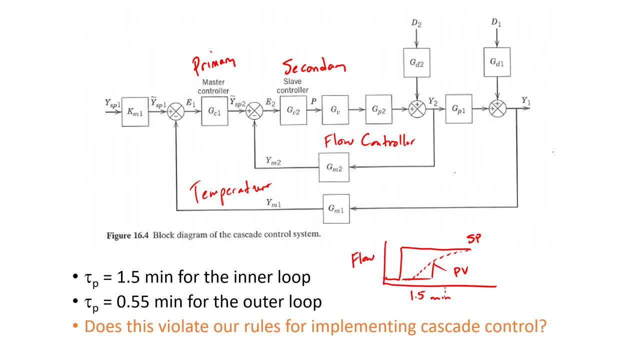 faster, so I tune it to get there in about 0.5 minutes. So does this violate our rules for implementing cascade control? So the answer is yes, because this is too aggressive. The outer loop is going to be asking for something to change. 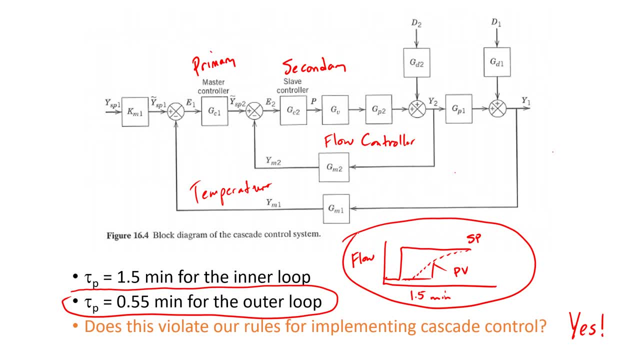 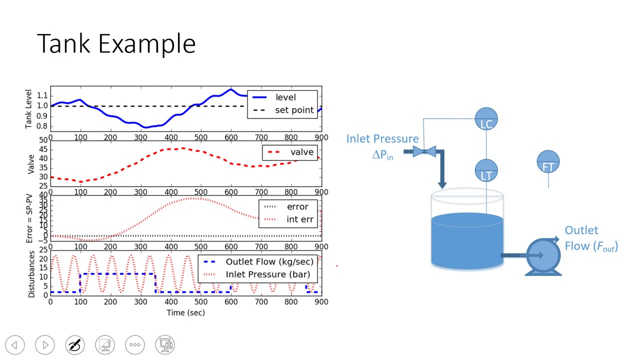 much faster than the inner loop can actually change it. So that's going to result in things like instability of this cascade controller. Here's a tank example- just one last example here- where we're trying to maintain a level in our tank and so we set up a level controller that then writes a valve position. 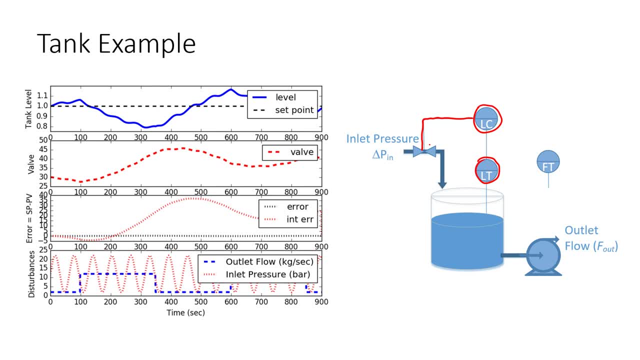 to an inlet flow. Now there's a couple disturbances that are affecting our system here. One is the outlet flow is going to change randomly as an operator turns on or off this pump. Another disturbance is that we have an inlet pressure fluctuation that's going to change over time. 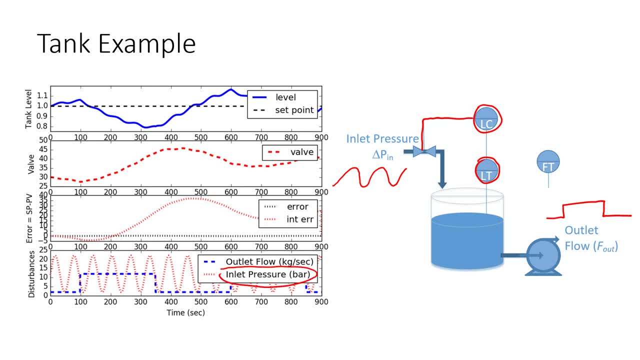 And you can see that right down here. with the inlet pressure changes And then we also have the outlet flow, It changes as well, And you can see that these disturbances are driving us away from our set point. So the little oscillations that you can see here, 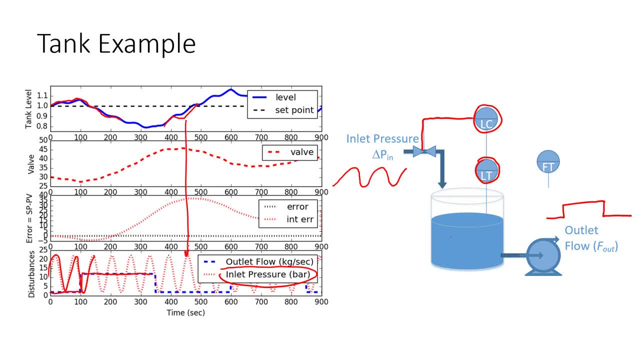 those are due to the pressure changes And the much longer period oscillations. those are due to my outlet flow, So somebody bought a flow transmitter for us, And so we want to install this in a way that will help us reject the disturbances and give us a cascade controller. 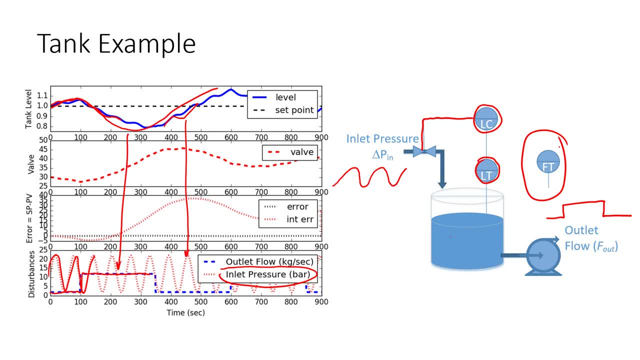 So where would we install that? To set up a cascade control system? Okay, so go ahead and pause the video right now and we'll talk about this for a little bit, And then we'll start again in just a second. Okay, so what we're going to do for this?